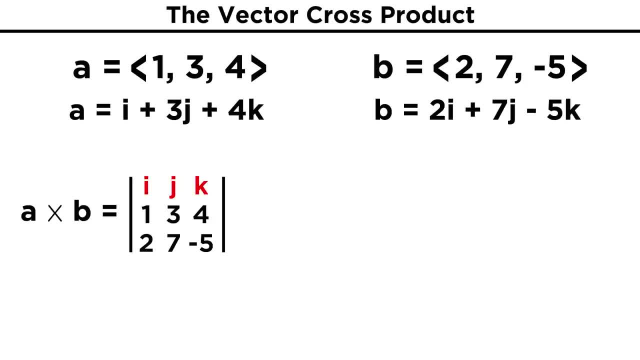 of the following three by three matrix, with I, J and K across the top row, the components from vector A in the second row and the components from vector B in the third row. We know how to get the determinant of a three by three matrix, so this is no problem. 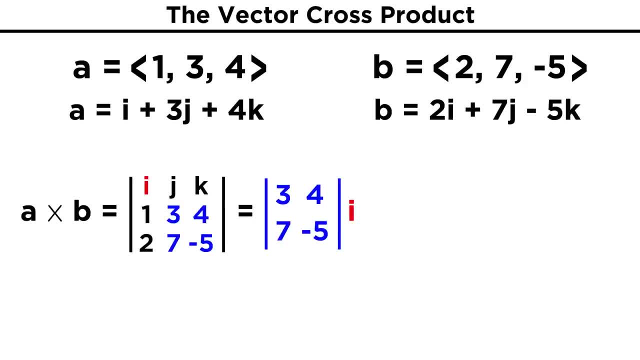 We just get. I times the determinant of this two by two: matrix minus J times the determinant of this one, plus K times the determinant of this one. Now we can find each of these determinants. First we have negative fifteen minus twenty-eight, then negative five minus eight and then seven. 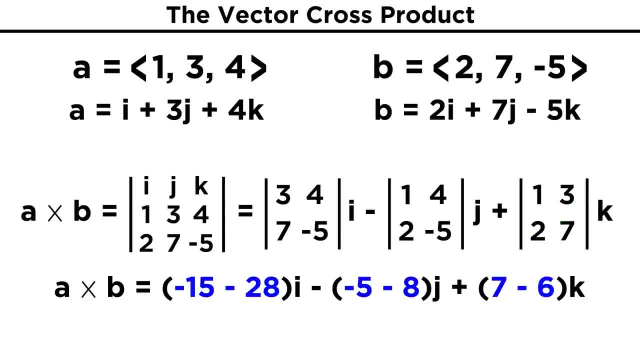 minus six. Simplifying and combining with the unit vectors, we are left with negative forty-three I and then seven minus six. So we can see how, using determinants, we have found the cross product of these two vectors, which is another different vector. 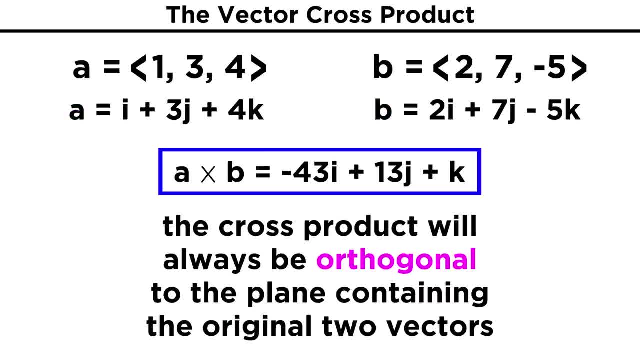 We must understand that a vector cross product will always yield a vector that is orthogonal or perpendicular to the original two vectors, or rather to the plane containing them. In fact, if you place the edge of your right hand directly on vector A, then the vector 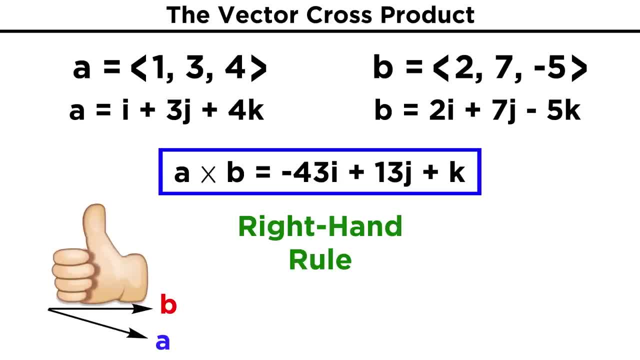 B and curl your fingers in the direction of vector A so that your hand is sort of mimicking the angle formed between them. your thumb will be pointing in the direction of their cross product. Alternately, you can point your index finger in the direction of A and your middle finger. 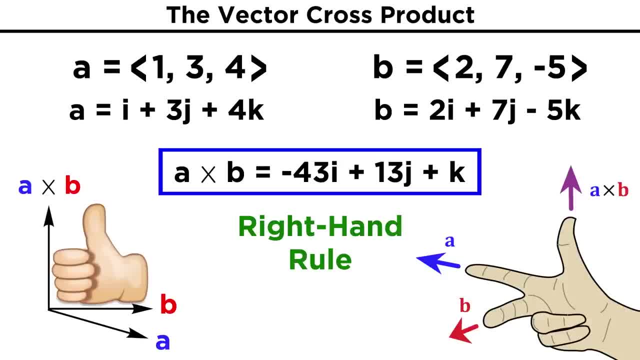 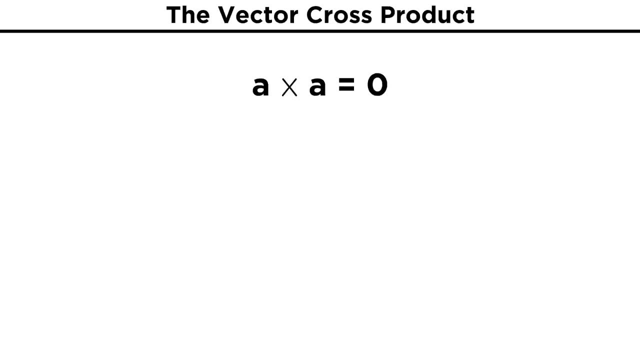 in the direction of B, and again your thumb will be pointed in the direction of the cross product. So the right hand rule that we originally learned for three-dimensional coordinate systems can help us understand the direction of a cross product. There are a few other key points to understand about cross products. 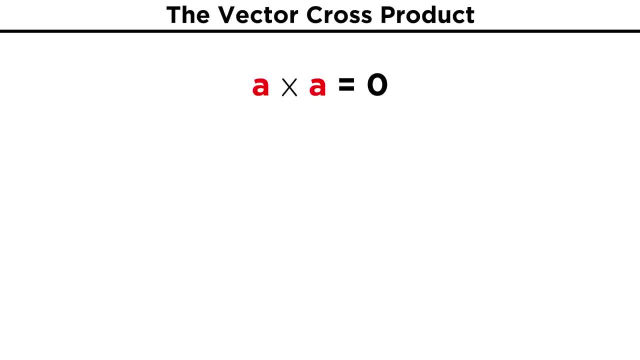 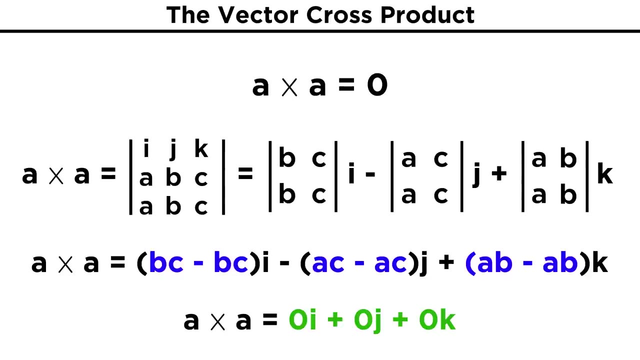 First, if you take the cross product of a vector and itself like A cross A, you will always get zero. This will be easy to prove to yourself if you work out the determinant, just as we did before, and see that all the terms cancel out. Simplifying and combining with the unit vectors, we are left with negative forty-three I, and then seven minus six. 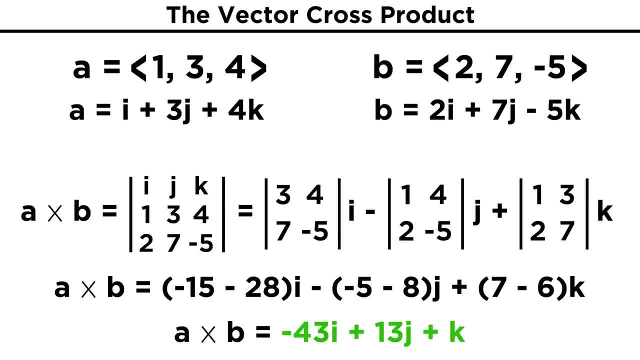 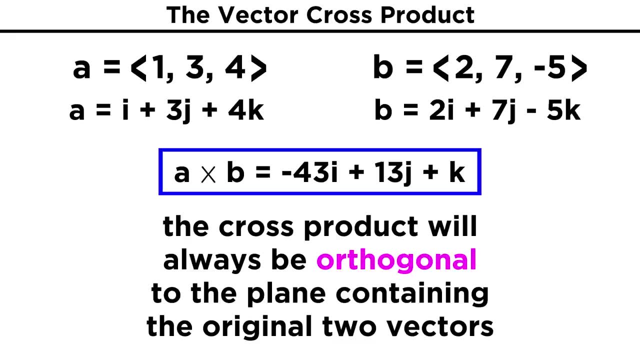 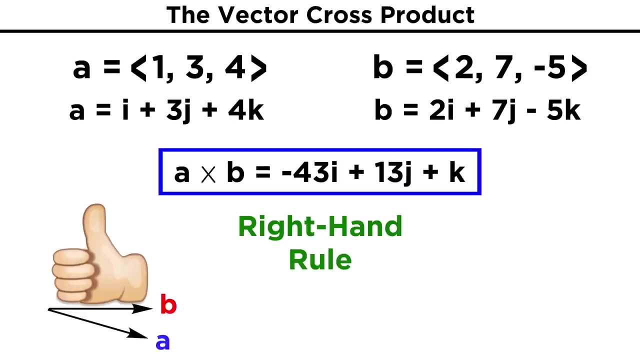 So we can see how using determinants, we have found the cross product of these two vectors, which is another, different vector. We must understand that a vector cross product will always yield a vector that is orthogonal, or perpendicular, to the original two vectors, or rather to the plane containing them. In fact, if you place the edge of your right hand directly on vector A, then the vector B, and curl your fingers in the direction of vector A so that your hand is sort of mimicking the angle formed between them, your thumb will be pointing in the direction of their cross product. 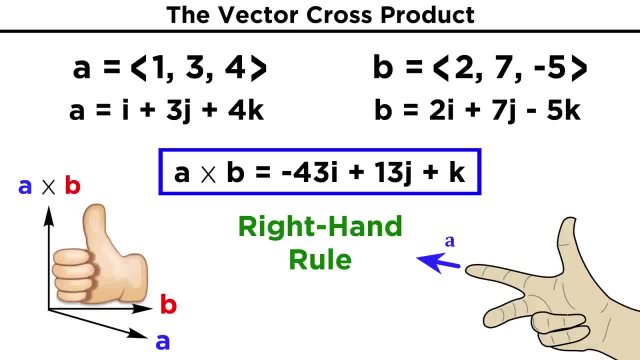 Alternately, you can point your index finger in the direction of A, and your middle finger in the direction of B, and again your thumb will be pointed in the direction of the cross product. 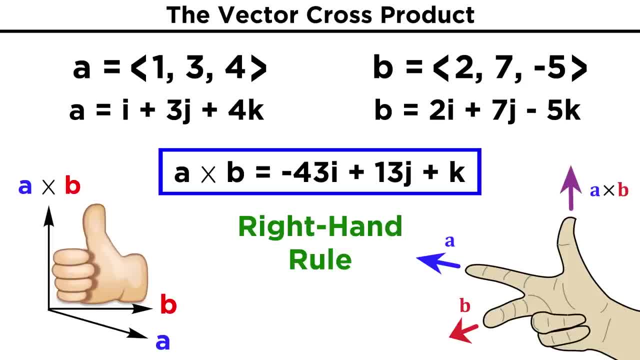 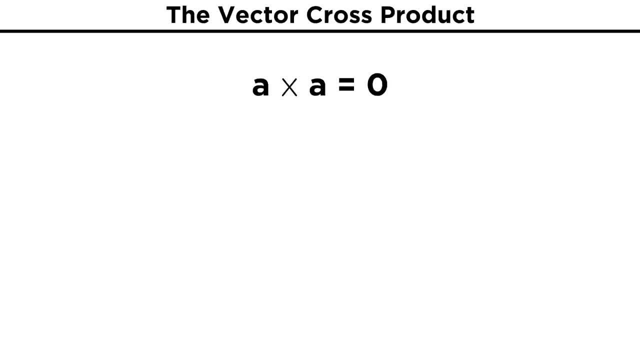 So the right hand rule that we originally learned for three-dimensional coordinate systems can help us understand the direction of a cross product. There are a few other key points to understand about cross products. 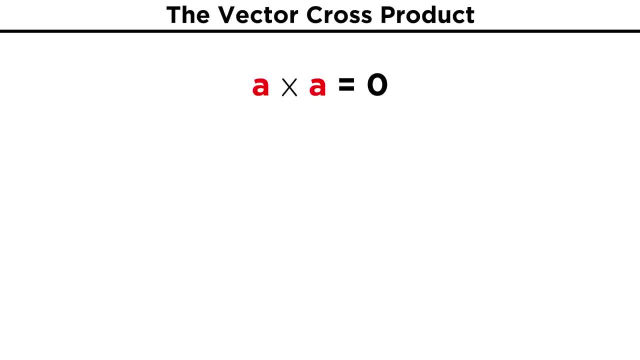 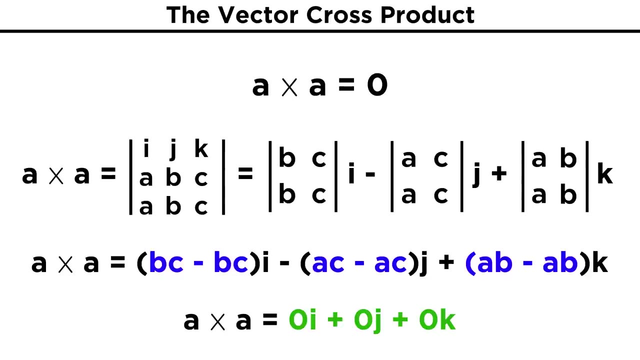 First, if you take the cross product of a vector and itself, like A cross A, you will always get zero. This will be easy to prove to yourself if you work out the determinant just as we did before and see that all the terms cancel out. Also, if you take the vector itself, you will always get zero. This will be easy to prove to yourself if you work out the determinant just as we did before and see that all the terms cancel out. 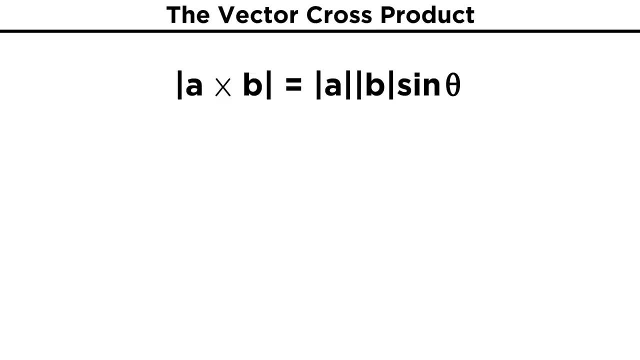 Also, we can make the following statement about the length of the cross product vector. the magnitude of A cross B is equal to the magnitude of A, times the magnitude of B, times the sine of the angle between them. This definition can also be used to find the cross product of two vectors, because magnitude and direction are the two pieces of information conveyed by any vector. And if we calculate the magnitude of the cross product this way happen side by side, you will definitely get this right. 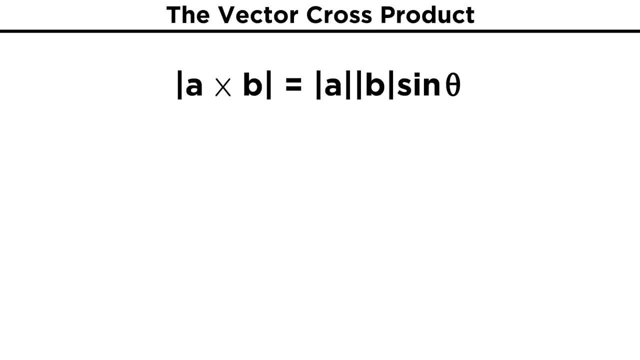 Also, if you take the vector itself, you will always get zero. This will be easy to prove to yourself if you work out the determinant, just as we did before, and see that all the terms cancel out. Also, we can make the following statement about the length of the cross product vector: 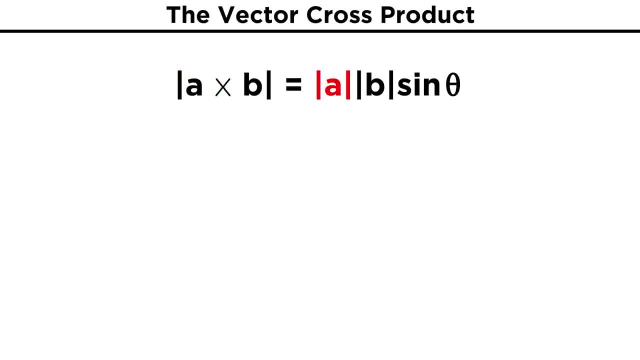 The magnitude of A cross B is equal to the magnitude of A times the magnitude of B times the sine of the angle between them. This definition can also be used to find the cross product of two vectors, because magnitude and direction are the two pieces of information conveyed by any vector, and if we calculate, 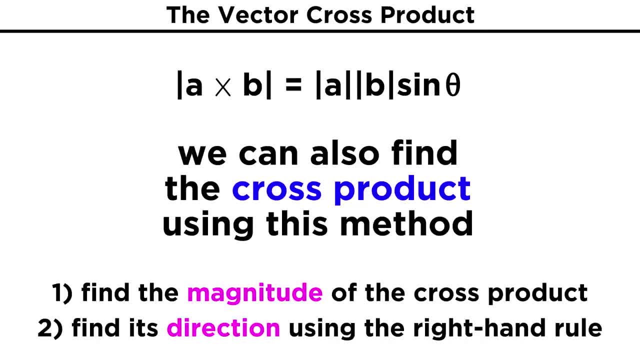 the magnitude of the cross product this way and then determine the length of the cross product. we will be able to find the length of the cross product If we can determine its direction by using the right-hand rule. we can therefore accurately define this cross product. 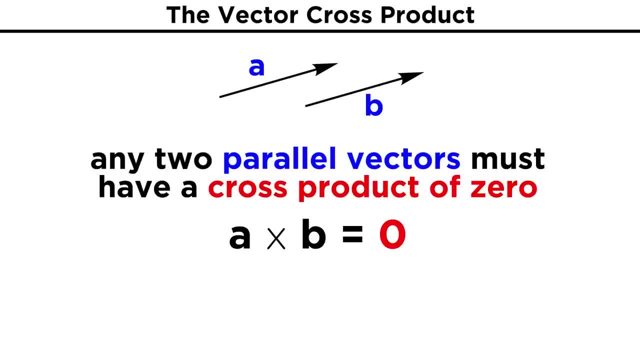 From this method we can also arrive at another truth: that any two parallel vectors must have a cross product equal to zero. That's because parallel vectors have an angle of zero between them and the sine of zero is zero. so the whole cross product, according to this expression, must go to zero. 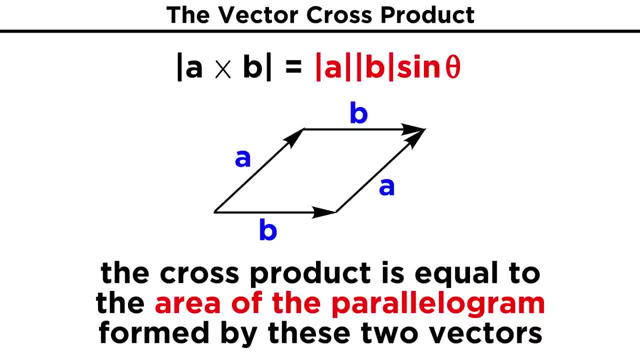 When we look at the cross product of two vectors, we see that the length of the cross product is equal to zero. One other interesting thing about the cross product is that the magnitude of the resulting vector, which is the AB sine theta expression we just used, will also be equal to the area. 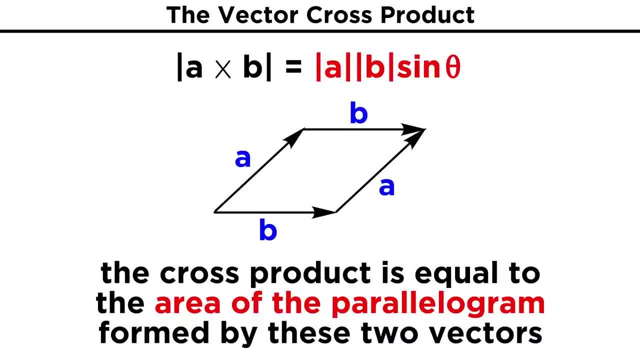 of the parallelogram created by vectors A and B. This is another reason that the cross product of parallel vectors is the zero vector, because they span zero area. Lastly, just as we learned some properties of the dot product, let's quickly mention: 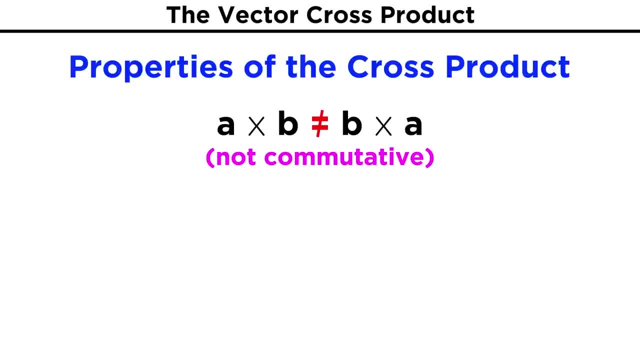 some properties of the cross product. First, the cross product is not commutative. A cross B does not equal B cross A. Rather, A cross B equals negative B cross A. Second, the cross product is not associative. The quantity A cross B cross C is not equal to A cross the quantity B cross C. However, 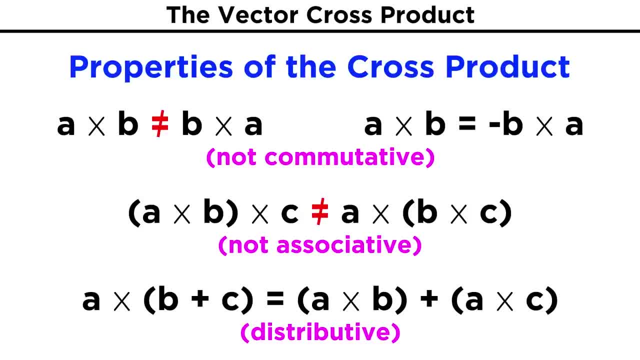 the cross product does distribute A cross, the quantity B plus C is equal to A cross B plus A cross C. This understanding of the cross product will suffice for our purposes, and we should note that the cross product crops up all the time in physics. but let's keep going with linear algebra. 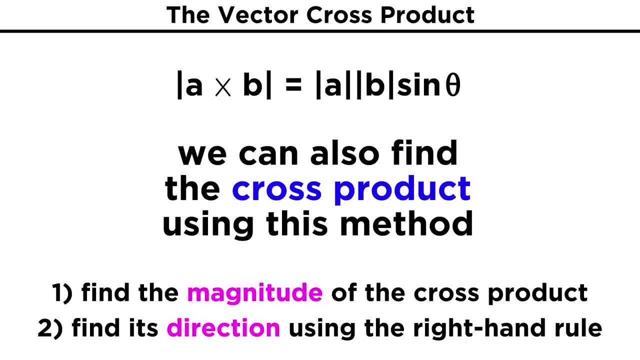 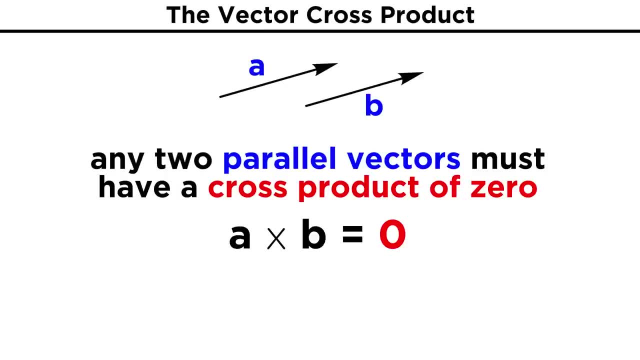 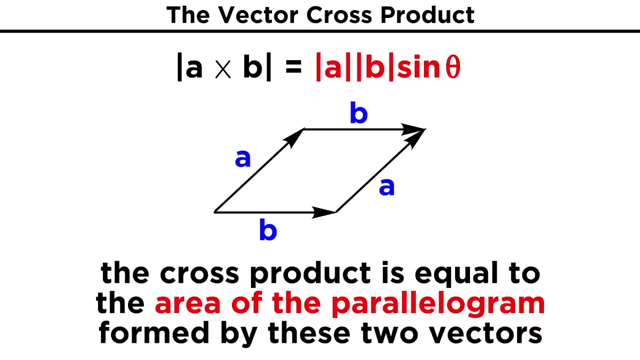 its direction by using the right-hand rule, we can therefore accurately define this cross-product. From this method we can also arrive at another truth, that any two parallel vectors must have a cross-product equal to zero. That's because parallel vectors have an angle of zero between them, and the sine of zero is zero, so the whole cross-product, according to this expression, must go to zero. One other interesting thing about the cross-product is that the magnitude of the resulting vector, which is the AB sine theta expression we just used, will also be equal to the area of the parallelogram created by vectors A and B. This is another reason that the cross-product of parallel vectors is the zero vector, because they span zero area. 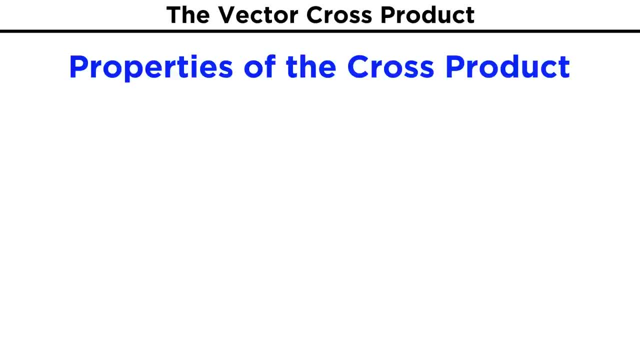 Lastly, just as we learned some properties of the dot product, let's quickly mention some 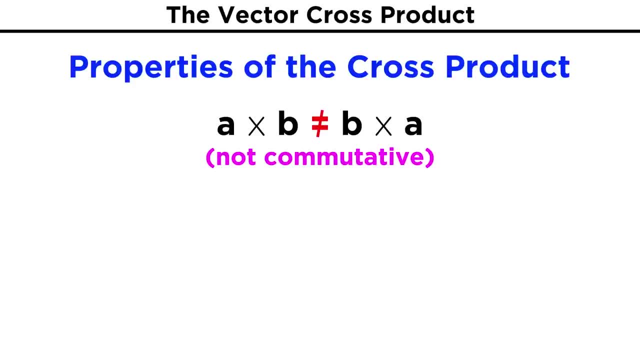 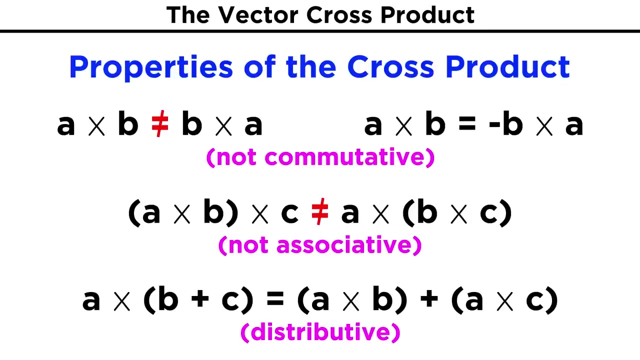 properties of the cross product. First, the cross product is not commutative. A cross B does not equal B cross A. Rather, A cross B equals negative B cross A. Second, the cross product is not associative. The quantity A cross B cross C is not equal to A cross the quantity B cross C. However, the cross product does distribute. A cross the quantity B plus C is equal to A cross B plus A cross C. This understanding of the cross product will suffice for our purposes, and we should note that the cross product crops up all the time in physics, but let's keep going with linear algebra right after we check comprehension. 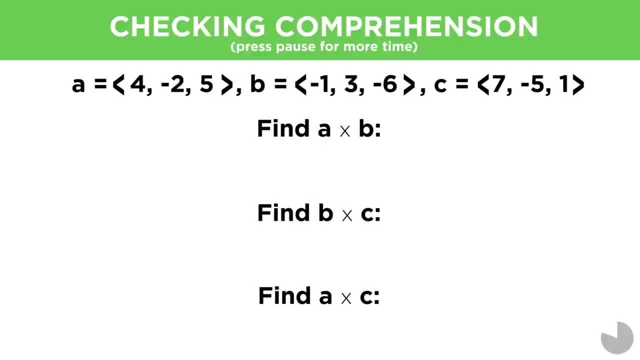 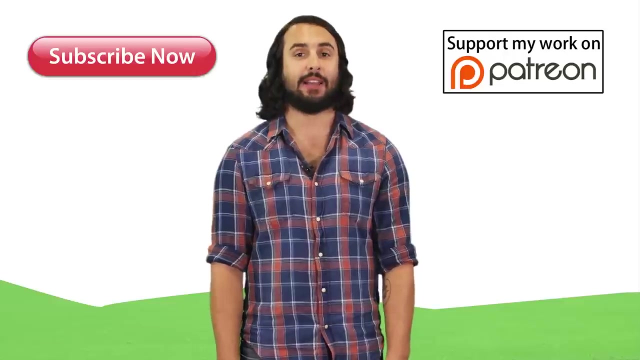 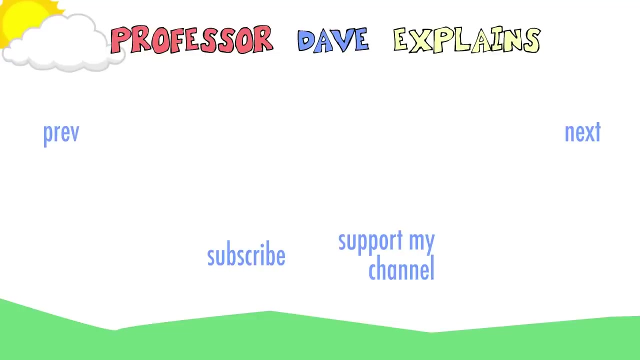 Thanks for watching, guys. Subscribe to my channel for more tutorials. Support me on Patreon so I can keep making content. And as always, feel free to email me, professordaveexplains at gmail dot com. I'll see you in the next video. Bye!